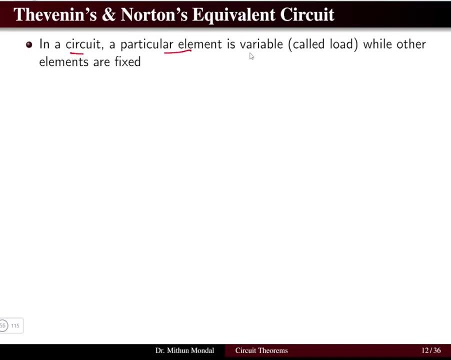 a circuit will have a particular element which is variable in nature- that is known as the load- while the other elements are fixed. So in a complex circuit there will be having a lot of elements which are fixed, which are not variable, whereas a particular element may be variable. that 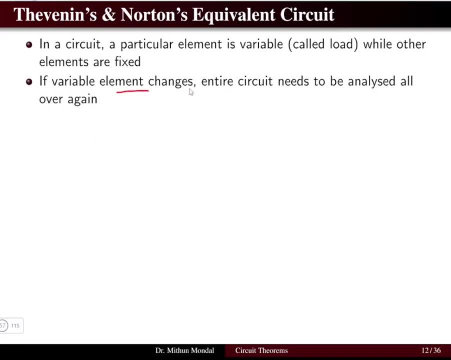 is known as the load. If the variable element changes, the circuit need to be analyzed all over again. So due to the changes of the load, that is, the resistance of the load, the entire circuit need to be analyzed All over again. So if this is detached from the fixed element, then the circuit analysis would 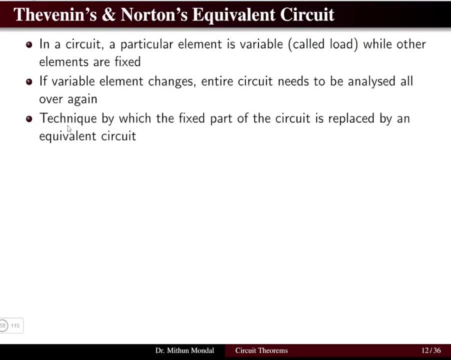 have been much easier. So we are going to study some technique by which the fixed part of the circuit is replaced by an equivalent circuit. So in a circuit we will replace the fixed part with the variable part. The fixed part will remain constant and the variable part can change. 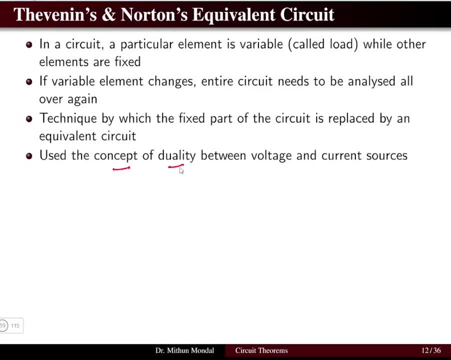 We will use this concept based on the duality principle, That is, the voltage and the current source are dual of each other, So the technique by which we transform the fixed part of the circuit into its equivalent circuit is based on the principle of. 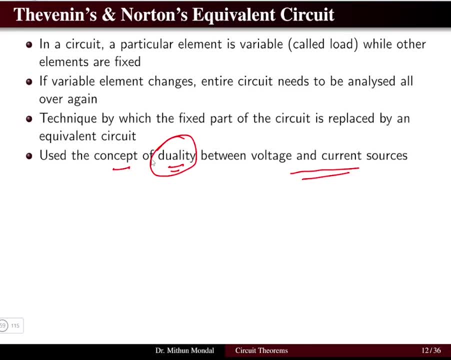 duality, where the voltage and the current source can be converted from one to another. Now let us see with the help of a diagram. So in a circuit, our load, which is a part of the circuit, is variable, Whereas the linear two-terminal circuit is basically that part of the circuit which is fixed. 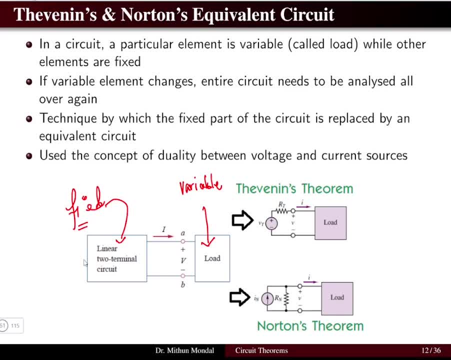 So this part of the circuit can be as complex as possible. So this can be very complex in nature. The load is variable, which can change, and on changing the entire dynamics of the circuit will change. So we detach this part of the circuit and keep the fixed part of the circuit to form an equivalent part. 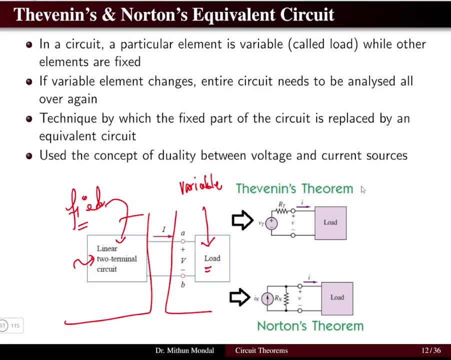 This can be done using two theorems. One is known as the Thevenin's theorem and another is known as the Norton's theorem, So the fixed part of the circuit if it is replaced with a single voltage source in series with a resistance. it is known as the Thevenin's theorem. 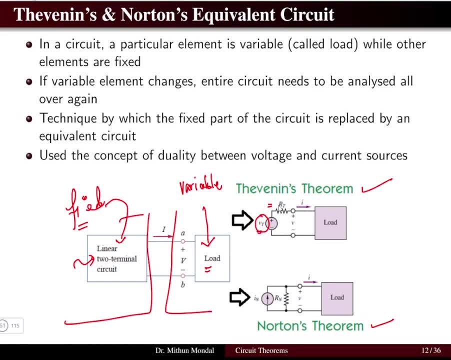 The voltage source is known as the Thevenin's voltage and the series resistance is known as the Thevenin's resistance, The load is at the terminal of the circuit. Similarly, if the fixed part of the circuit is replaced with a current source in parallel with a resistance, 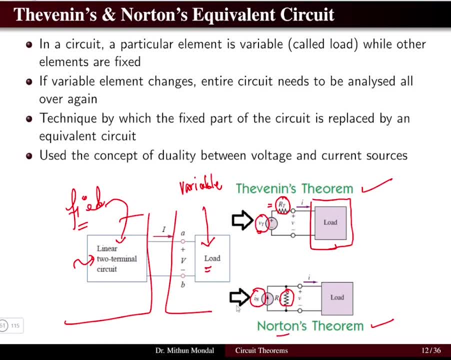 then this is in accordance with the Norton's theorem, where the current source is known as the Norton current and the resistance is known as the Norton resistance. The load is again at the terminal. So these two circuits are one and the same, based on the principle of duality, where 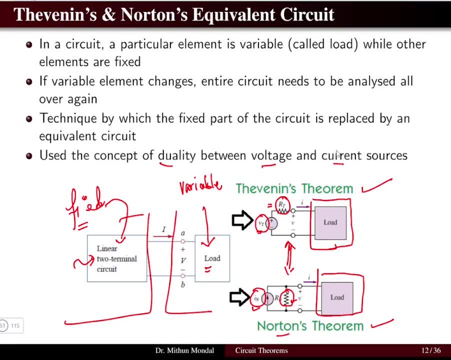 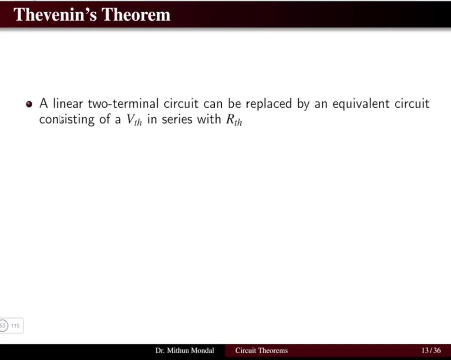 the terminal voltage and current relationship would remain the same. First we will study the Thevenin's theorem, then we will go for Norton's theorem. So what is a Thevenin's theorem? Thevenin's theorem states that a linear two-terminal circuit can be replaced by an. 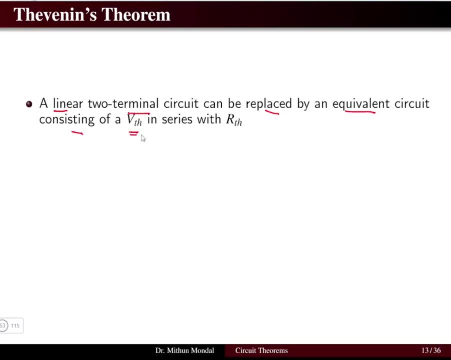 equivalent circuit consisting of a Thevenin voltage source in series with a resistance that is R Thevenin. The Thevenin voltage is the open circuit voltage at the terminal. So keeping the terminal open, that is, detaching the load, what is the voltage that is obtained at the terminal? 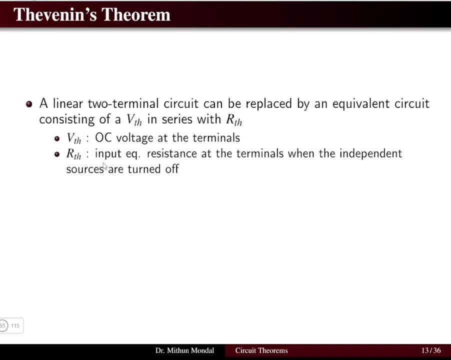 is known as the Thevenin's voltage. Similarly, the input equivalent resistance which is determined at the terminal when the independent sources are turned off. that is known as the resistance Thevenin resistance. So we have to determine voltage, Thevenin and Thevenin resistance. Then we 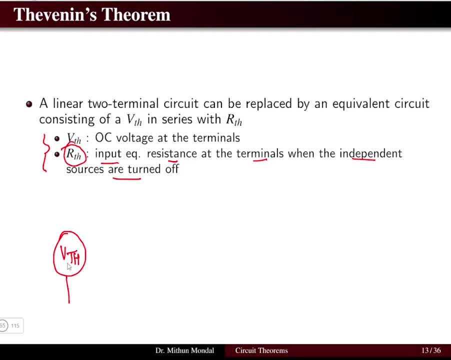 can form a circuit which is equal to a Thevenin's voltage in series with a resistance, Thevenin. This is known as the Thevenin's voltage. So that is the Thevenin's theorem. Now the terminal can have any load which is variable in nature. 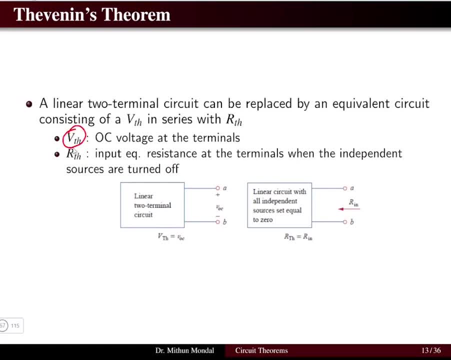 Now we have to obtain the Thevenin's voltage and Thevenin's resistance. So Thevenin's voltage is the open circuit voltage which is determined at the terminal, Whereas the resistance Thevenin is the input resistance which is determined at the terminal when 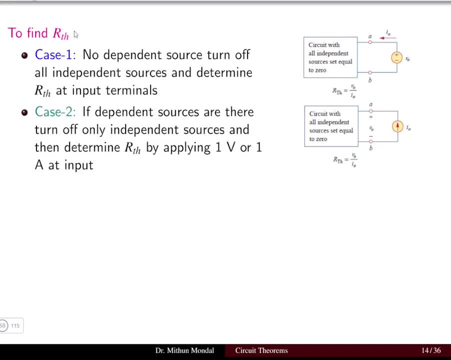 the independent sources are turned off. Now how to find the Thevenin resistance using two cases. Now how to find the Thevenin resistance using two cases, one and case two. First, let us take the case one, where no dependent sources are present. If there, 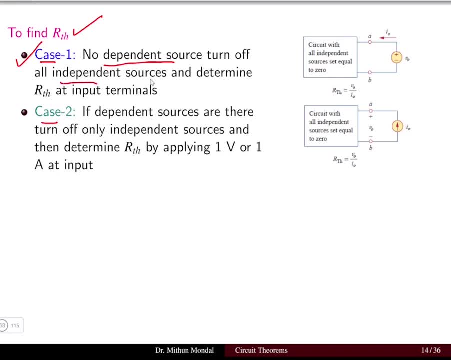 are no dependent sources, then all independent sources are turned off and we determine the resistance heavening at the input terminal, which is quite easy. So if dependent sources are not there, it is very easy to determine the earth heavening simply by removing all the independent sources and determining the resistance heavening at the input terminal. However, case two, if 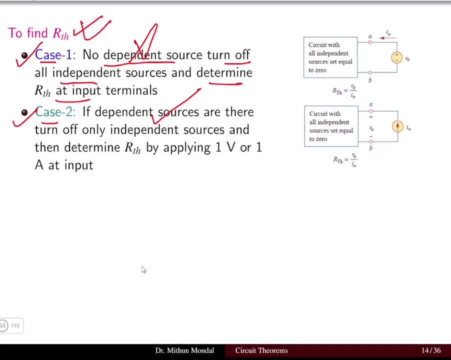 dependent sources are there, then what we do is that we turn off only the independent sources, whereas the dependent sources will be present in the circuit, and then, in order to determine the earth heavening, we apply one volt voltage source at the terminal or one ampere current source at 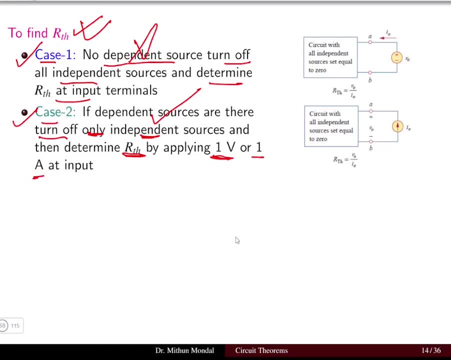 the input terminal. So we can determine the resistance heavening at the input terminal. So there are two different ways by which this can be determined. We can determine the value of earth heavening using a voltage source which is equal to one volt, which is connected at the 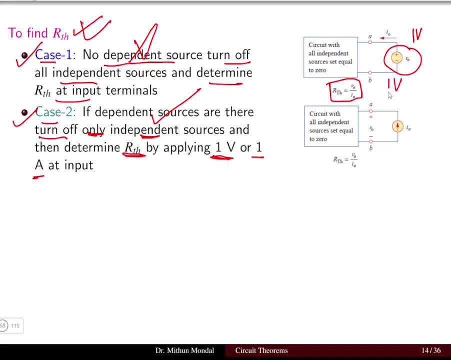 terminal. So earth heavening is equal to one volt divided by the current I naught which is coming out from the voltage source. So in this we need to measure what is the value of the current when the input is one volt. voltage source: This can be done by connecting the voltage source to the 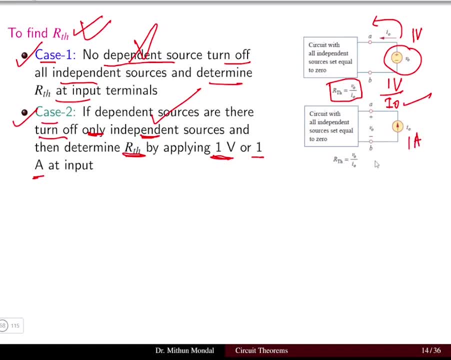 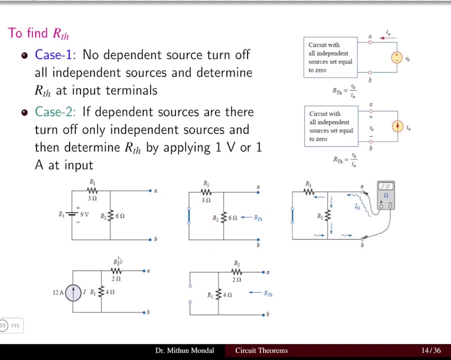 1 ampere current source at the input and determining the resistance using determining the voltage V naught by 1 ampere. So this is the reverse process of this. Both will give you the same result of the heavening resistance. Let us take one example where we have a voltage source. 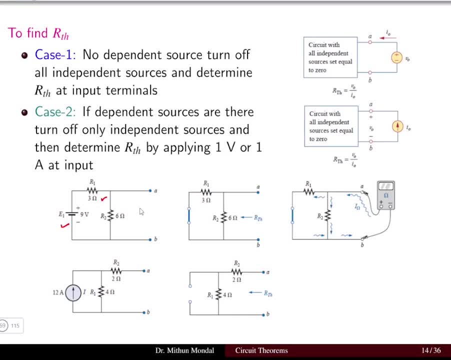 9 volt and there are two resistances, 3 ohms and 6 ohms. We need to determine the earth heavening here. So in order to determine the earth heavening, we short circuit the independent voltage source. So we have here, we have short circuited and we have determined the earth heavening, which is 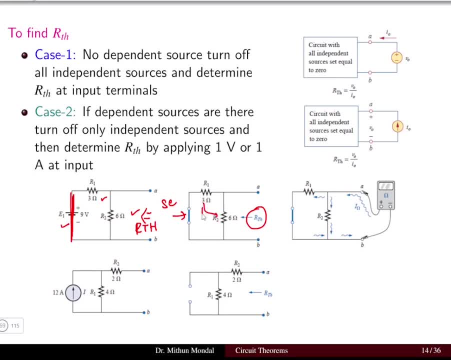 basically the parallel of these two resistances. Similarly, if we have a current source which is independent current source, then we have to open, circuit the independent source, keeping the other resistance constant, and then we need to determine what is the value of earth heavening. So this is the 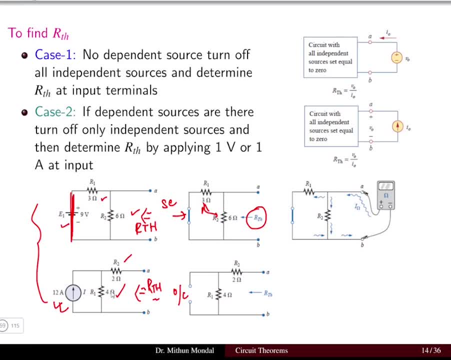 most simple way to understand the earth heavening, where the voltage source is convert, change to short circuit and the current source is changed to open circuit, because we have to remove the independent sources and then we have to measure the value of earth heavening using any technique here. So the technique can be most. 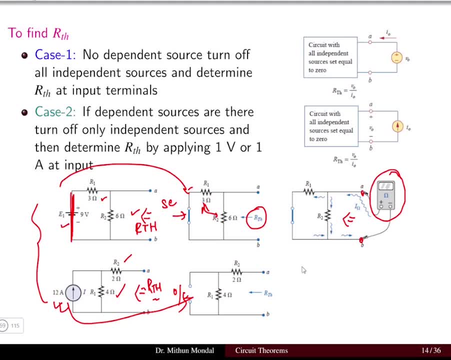 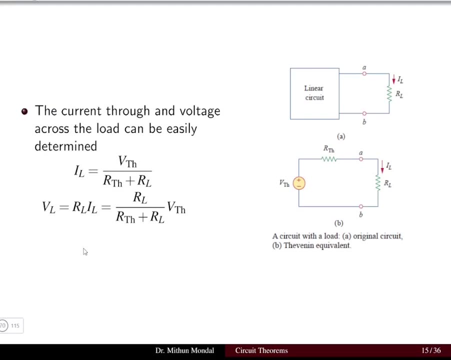 easily used to determine the earth heavening. So this is the way of determining the earth heavening. The example has been taken only for the independent sources. If dependent sources are there, we need not to remove the dependent sources, only independent sources. we need to remove Now the benefit of 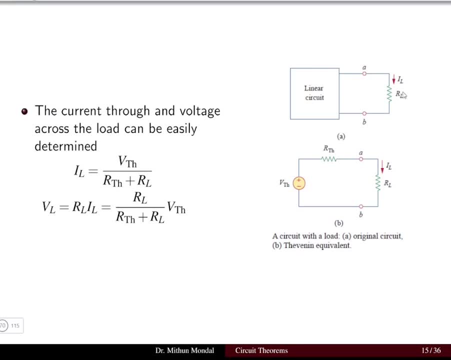 obtaining the equivalent circuit is the load register where the current iL is flowing due to the variable load register RL. What is happening is that the load register RL is being moved to the. the current which is flowing in the load register will change with a change in the resistance. 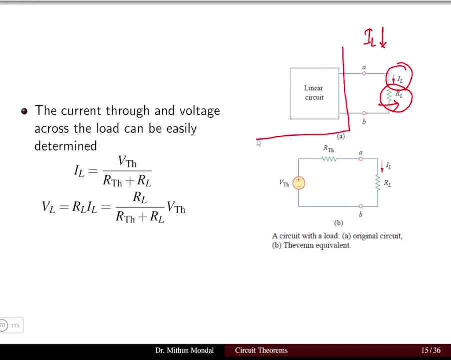 So if we detach the rest part of the circuit from the variable part, then we can obtain a circuit which is much simpler of the previous version. So we will have a Thevenin's voltage in series with a Thevenin resistance, and this register can be variable. 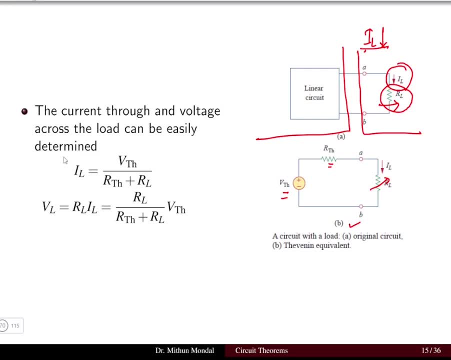 So for a particular RL the load voltage is equal to the total voltage, ie the Thevenin's voltage divided by the total resistance, R equivalent. So R equivalent is the series combination of R? Thevenin plus RL. So R? Thevenin plus RL will give you R equivalent. 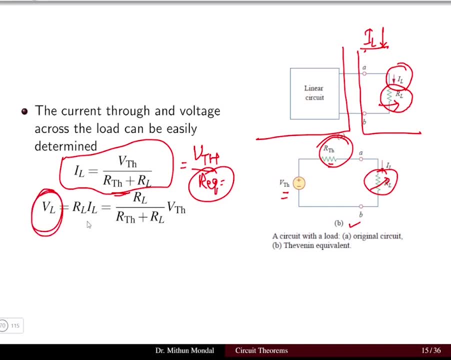 Similarly, the voltage of the load is equal to the load current multiplied with the load resistance. And load current we can substitute from the previous equation. So we can see that the linear Zito change in the load register. the circuit would have become more complex and more number of iterations. 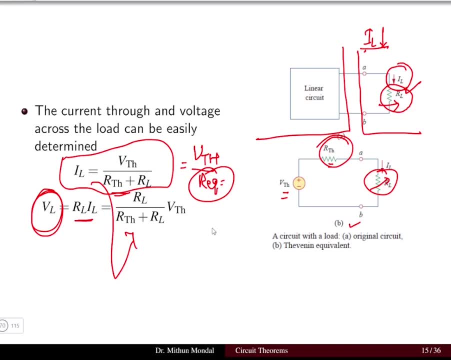 we could have done in solving the circuit. But if we detach the fixed part of the circuit and keep that constant with a Thevenin's voltage and Thevenin's resistance part, then whatever may be the changes happening at the load of the variable part, we can easily determine that. 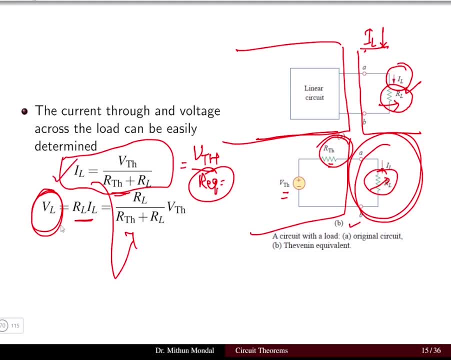 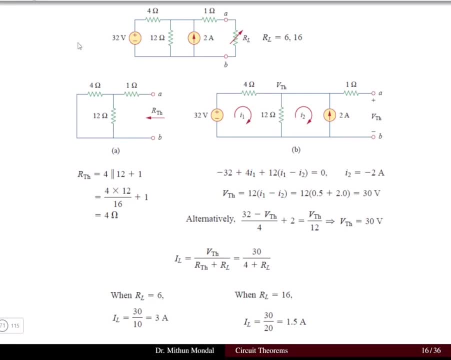 using the basic formula of the current and the voltage. So we'll solve one example of Thevenin's voltage. So our original circuit looks like this: We have a 32 volt voltage source, 2 ampere current source and there are too many registers: 4 ohms, 12 ohms, 1 ohms. 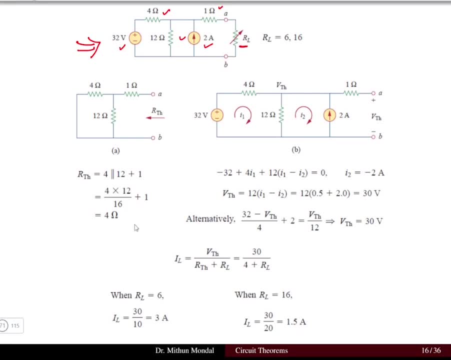 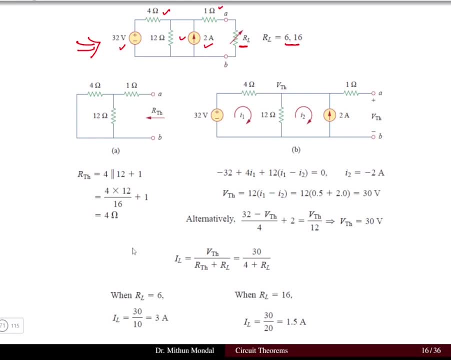 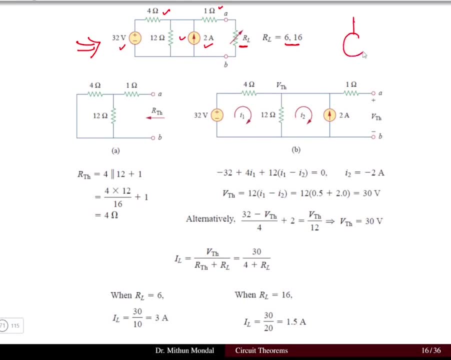 So in Thevenin we basically required a single voltage source, which is basically the Thevenin's voltage in series with a Thevenin's resistance, R Thevenin, and at the terminal, whatever the load will be there, that can be variable. 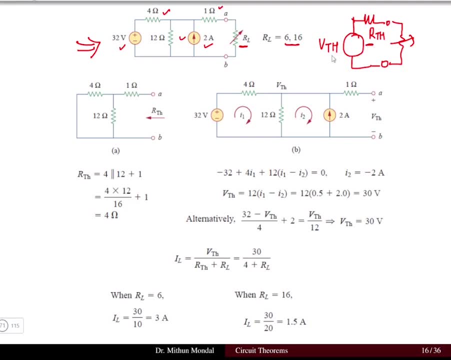 So our first aim would be to determine the R Thevenin and V30.. So let us determine the R Thevenin and V30.. To determine the R Thevenin first. we know that to determine the R Thevenin, all the independent. 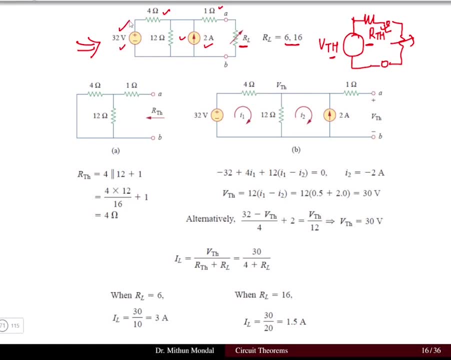 sources are turned off. So we have 32 volt independent source and 2 amp current source independently. So the voltage source will be replaced by short circuit and current source will be replaced by open circuit In order to do that. and we read where the 32 volt is short circuited here and the current 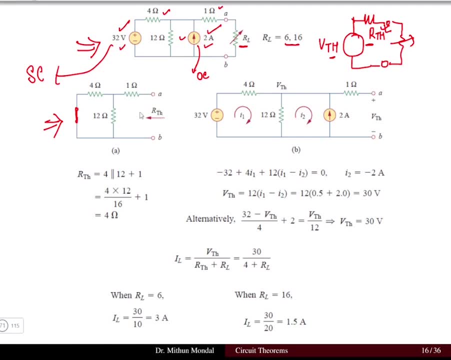 source, which was 2 ampere, is detached from the circuit and it is an independent part. So here we have an open circuit, So no current is flowing. So we have 4 ohm register here, 12 ohm in parallel. 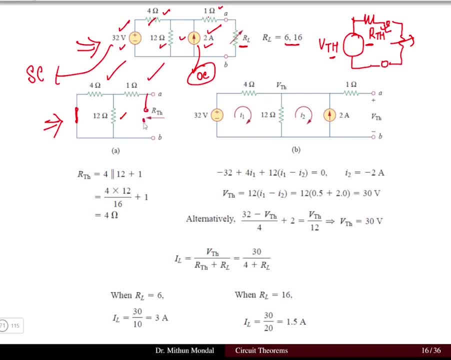 and 1 ohm will come here because this is open circuit. Now, in order to determine the Arthabin, we will use the series parallel concept of determining the equivalent resistance, where 4 ohm and 12 ohm are in parallel and the net is equivalent with the series of 1 ohms. So 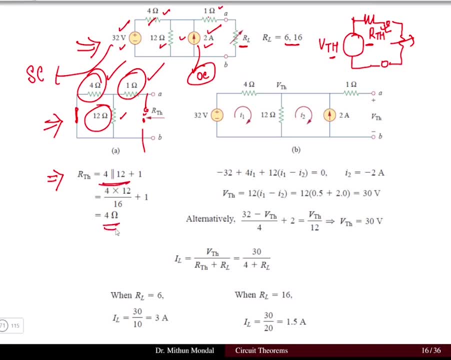 that is what we have done here: to determine the Arthabin, that is, 4 ohms. Now, having determined the Arthabin as 4 ohms, we will determine the voltage Thabin. Voltage Thabin is the voltage which is at the terminal A. So these can be determined by different method. We have shown: 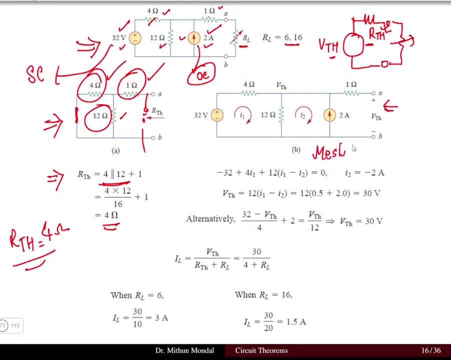 here two different methods. One is known as the mass analysis and other than nodal analysis. We can apply any analysis to determine the K-means voltage. So if we take two different loops, 1 and 2, and write down the equations, we can determine what is the voltage that is flowing through the 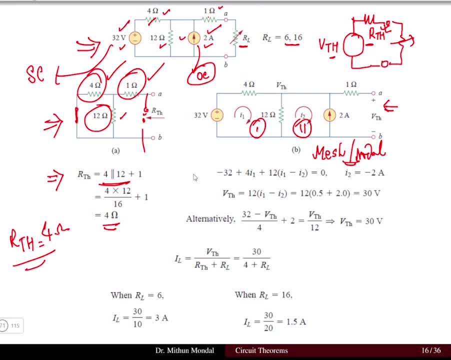 2 ohm current source. So the first equation that we need to write for the mass 1 is the K-mean equation In the mass 1, and the K-mean equation in the mass 2 need not be written because the current is at the boundary. So that gives you minus 2 ampere as the current because the direction 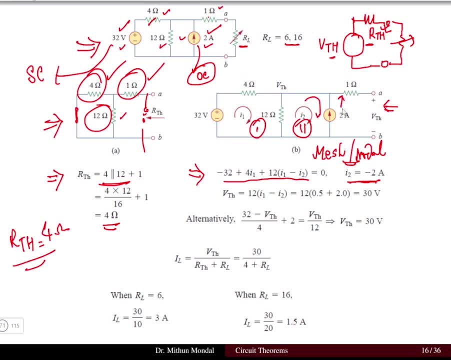 of the I2 variable is downward and 2 ampere is upward, So we have put a negative sign here. So the K-means voltage, which is the voltage at the terminal, is basically the 12, that is, the resistor multiplied with I1.. 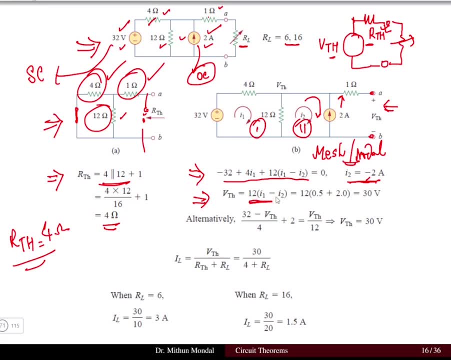 We can compute this voltage as I1 minus I2, because the current which is flowing is I1 minus I2. that will give you the 30 volt. So these K-means voltage can be obtained using the pulling circuit of this one. So we have 12 ohms where voltage K-mean is appearing. 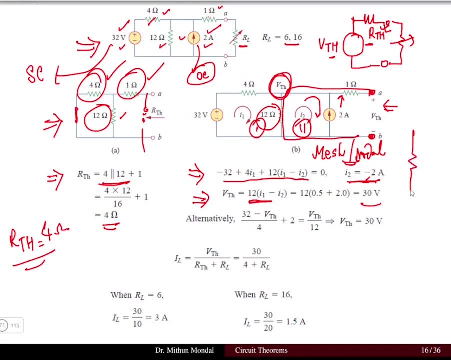 So the current that is flowing in 12 ohm register. I1 current is downward and I2 current is downward current is upward. So this is your I1 and this is your I2 and here you have 12 ohms. So 12 multiplied. 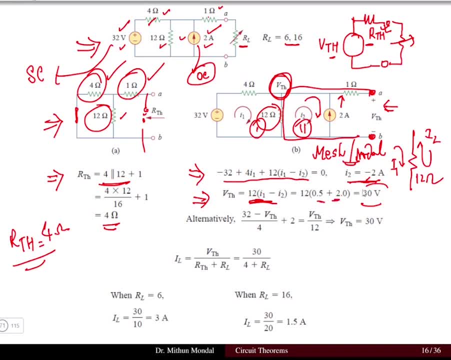 with I1 minus I2, putting the value of I1 and I2, we get 30 volt as the Thevenin's voltage. So this is determined with the help of mass analysis. We could have done using alternative method of nodal analysis too, to determine the Thevenin's voltage where the higher potential minus lower. 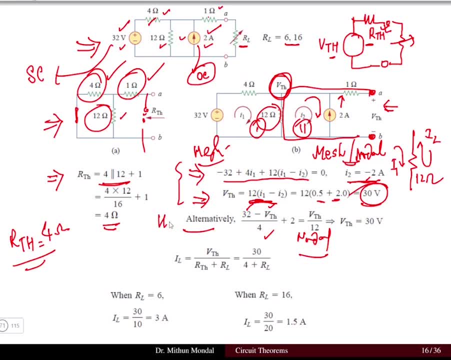 potential divided by the resistance, in accordance with Kirchhoff's current law, that is, the current entering is equal to current. leaving the circuit, we get the Thevenin's voltage as 30 volt. So we can see that whatever the technique we apply, whether it is a mass analysis or nodal analysis, 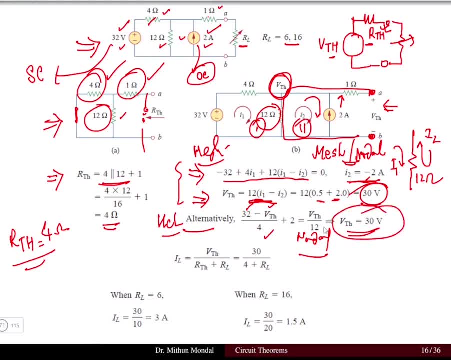 we reach to the same point, that is, the Thevenin's voltage is equal to 30 volt. Now we need to determine what is the current that is flowing in the load resistor IL when the resistance is changing from 6 to 16.. The current that is flowing? 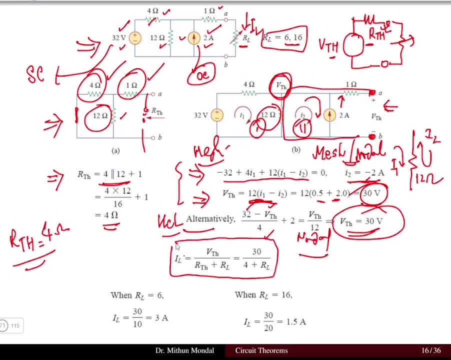 in the load resistor. IL is equal to the Thevenin's voltage divided by the total resistance, that is R Thevenin plus RL. So the Thevenin's voltage is 30 volt and the total resistance is 4 plus RL. We have kept the RL to be variable and we can put RL to be 6 ohms and RL to be 16 ohms. 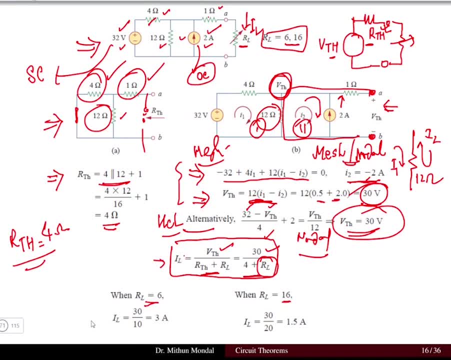 So by putting the value of RL we can get the current IL under two different cases of 6 ohms and 16 ohms. So we can understand from here that if the RL is changing and if this theorem is not applied, then the entire circuit need to be. 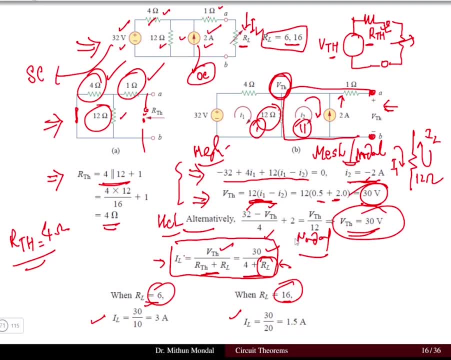 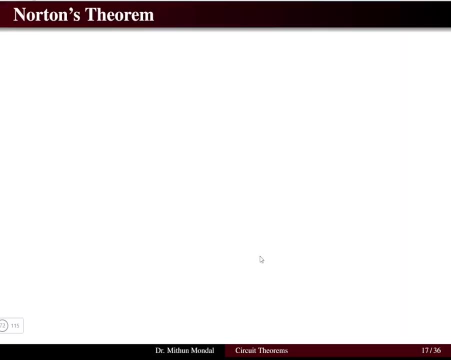 analyzed for all independent cases of RL. But since we have detached the variable part and the fixed part of the circuit, it was easy to calculate the current which is flowing through the load resistor IL. So that is the advantage of the Thevenin's theorem. Now we see the Norton's theorem. 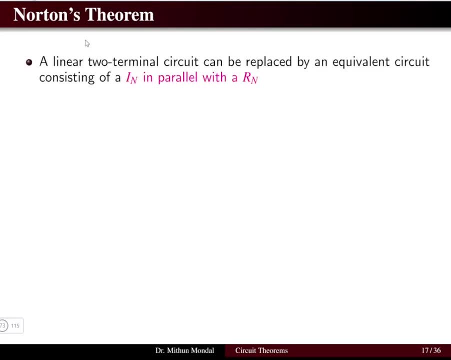 If we understand the Thevenin's theorem, it is very easy to see the Norton's theorem. The statements of the Norton's theorem is same. if we have a linear two terminal circuit, it will be replaced by an equivalent circuit. The equivalent circuit is such that the Norton current source is: 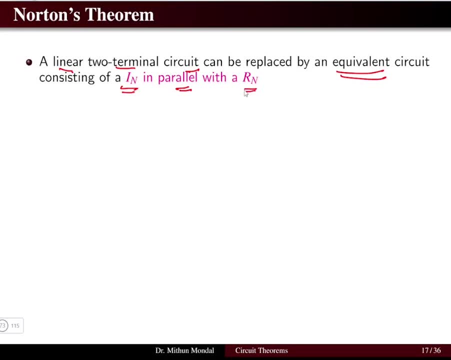 in parallel with a resistance, that is the R Norton. So in Thevenin's theorem we have the voltage Thevenin series with the R Thevenin. here we have the current, which is in parallel with R Norton. So we will see that how these Thevenin's and Norton's are related to each other. So the Norton current that we need. 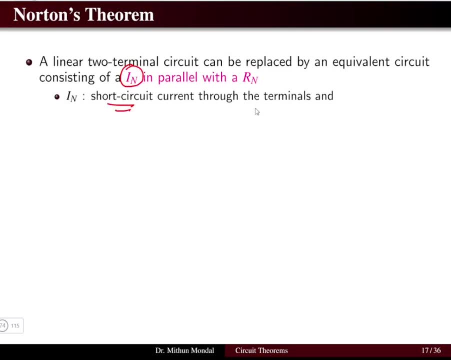 to determine is basically the short circuit current, which is determined through the terminals, and the R Norton is basically the resistance, which is the input equivalent resistance at the terminal when the input equivalent resistance is at the terminal. So the input equivalent resistance at the terminal means that the independent sources are turned off. So we will never turn off the. 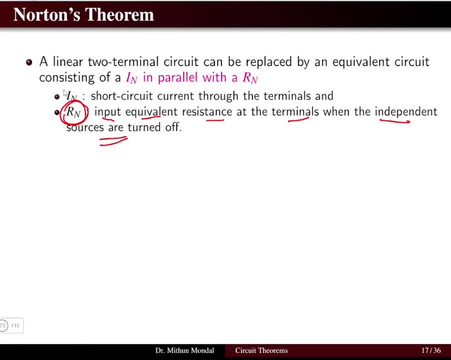 dependent sources, only the independent sources need to be turned off. So our aim of Norton's theorem would be to determine the value of I, N and R, N. So the circuit of any linear two terminal circuit, at the terminal A, B any variable load can be connected and this circuit has to be replaced. 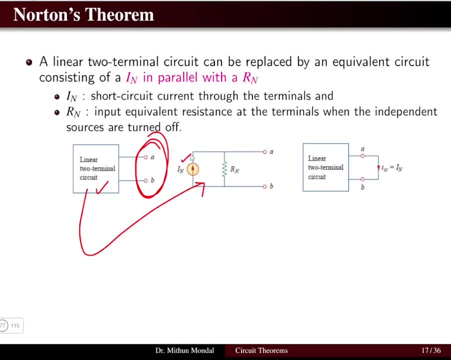 with a independent circuit where we have a Norton source in parallel with a resistance which is parallel with the Norton resistance and the Norton current is basically the short circuit current which is flowing through the terminals. If you remember, we have discussed that the Thevenin's 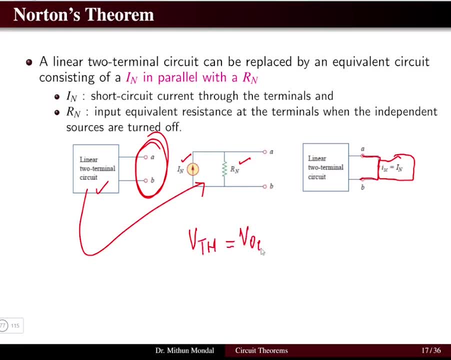 voltage is equal to the open circuit voltage at the terminal A. So here we have done. the Norton current is equal to the short circuit current which is flowing at the terminal A. That is the difference between the way by which you calculate the Thevenin's voltage and the Norton current. Now we can. 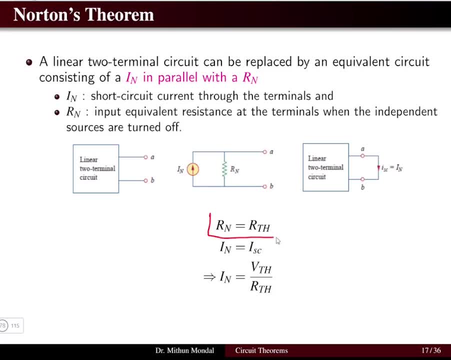 understand that the Norton resistance and the Thevenin resistance are one and the same, The Norton current and is equal to the short circuit current. So we can write: the Norton current relationship with the Thevenin's voltage is: the Norton current is equal to Thevenin's voltage. 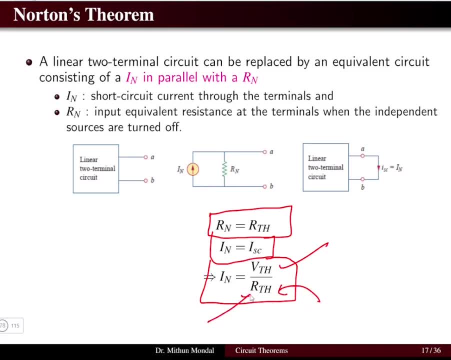 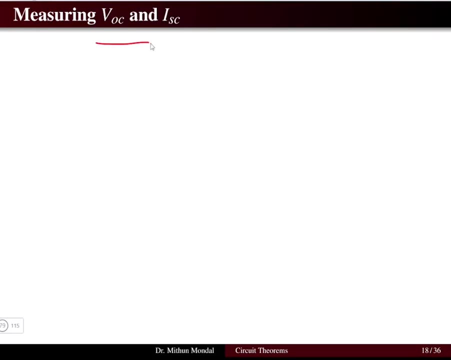 divided by Thevenin's resistance, Because Thevenin's resistance is equal to the resistance, and if we have already determined the Thevenin's voltage and the Thevenin's resistance, then it is easy to get the Norton current. Now how do we measure the open circuit voltage and 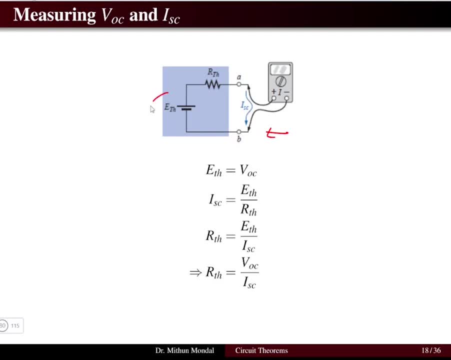 short circuit current. Let us take a circuit. we have the Thevenin's voltage, Thevenin's resistance and we have connected an emitter to measure the short circuit current. So the open circuit voltage is basically the Thevenin's voltage. The short circuit current we can see from the circuit is: 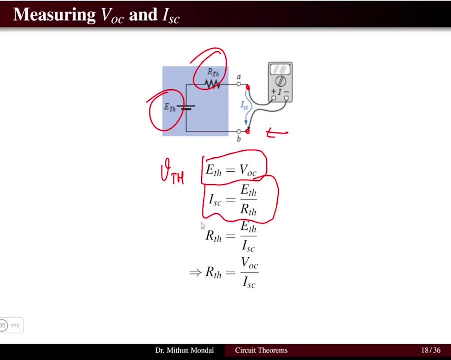 basically the Thevenin's voltage by Thevenin's resistance. So the Thevenin's resistance we can write as the ratio of Thevenin's voltage by short circuit current or the Norton current. Then the final conclusion is the Thevenin's resistance is open circuit voltage by short circuit current. 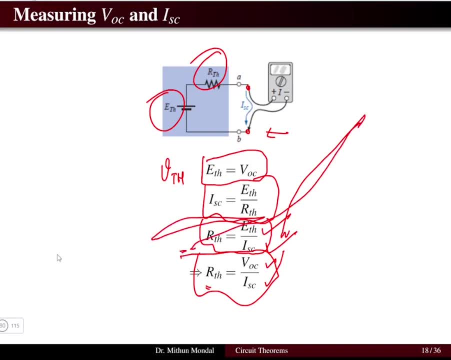 If you remember, we have basically solved: the Thevenin's resistance is equal to connection of one volt and one ampere current source at the terminal to obtain the Thevenin's resistance for a dependent sources. Same way we can do it here that the R Thevenin we can obtain as voltage open circuit by current short circuit. 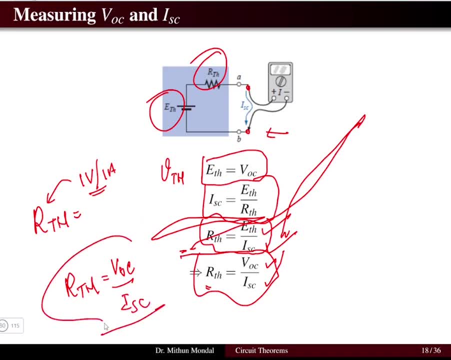 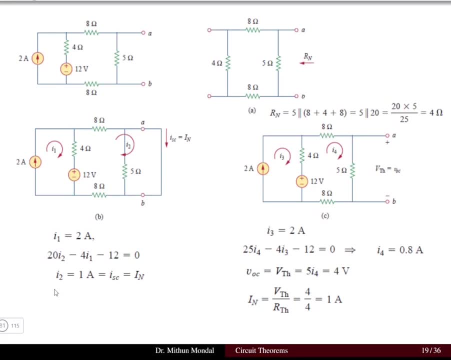 measuring at the terminal. So these all things, whatever calculation we are doing, we are doing at the terminals. Now we take one example for the Norton's theorem. Similarly what we understood from Thevenin's theorem, we will see the Norton's theorem. So this is our original circuit where we have a 2 ampere current. 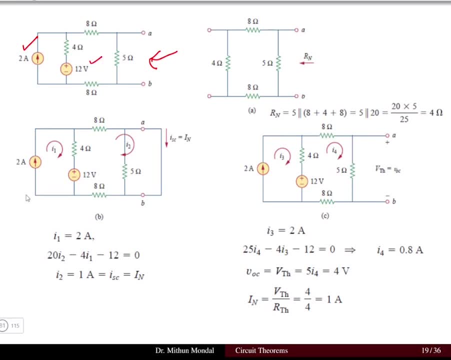 source that is independent, 12 volt voltage source, also independent, and we have some resistance which are connected in the circuit. We have to obtain a circuit which is I Norton- that is the current source- in parallel with one resistor That is R Norton, And here we have the terminal A and B. So how do we obtain this I Norton and R Norton for these circuits? 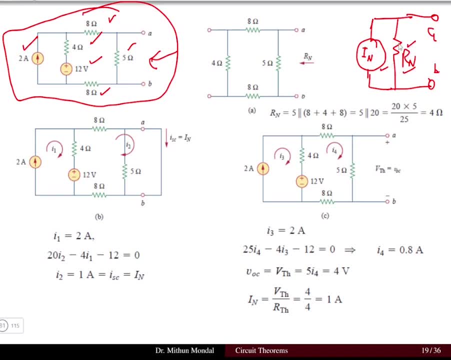 So we have discussed that R Norton and R Thevenin are equal and in order to determine that we have to replace all the independent sources by the open circuit or short circuit, depending upon whether it is a voltage source or a current source. voltage source: 12 volt will be short circuited and 2 ampere current source will be open circuited. 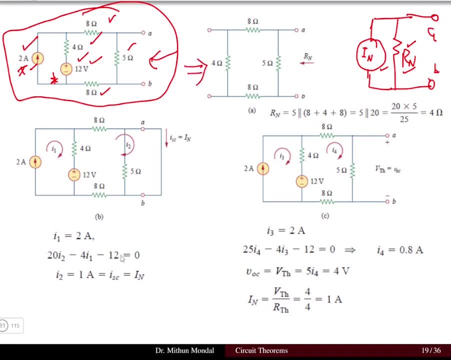 and we will redraw the circuit after removing the independent sources. Then we determine the R norton at the terminal, which is similar to what we have done for R3V. So, using the concept of series parallel, we get the R norton as 4 ohms. Now the second task is to get the I norton. I. 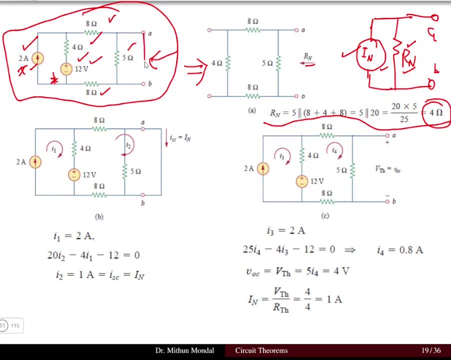 norton is basically the current which is flowing when AB- the terminal- is short circuited. So when the terminal is short circuited, what is the current flowing in the circuit? Now, to do that we have to apply some technique, earlier technique, whether it is a mesh analysis or node analysis. Here let us 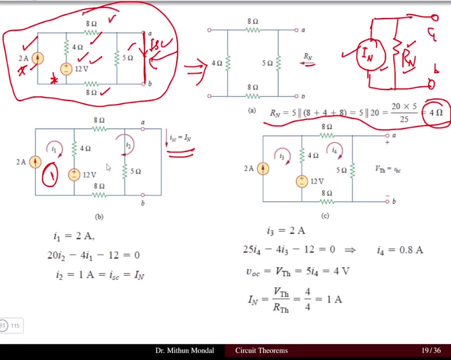 apply some mesh analysis technique. So we have mesh number 1, mesh number 2.. Now here we are basically sorting. So this part of the circuit is short circuited. So we have mesh number 1, mesh number 2 and the circuit will also be shorted because these two are parallel. The current I1, which 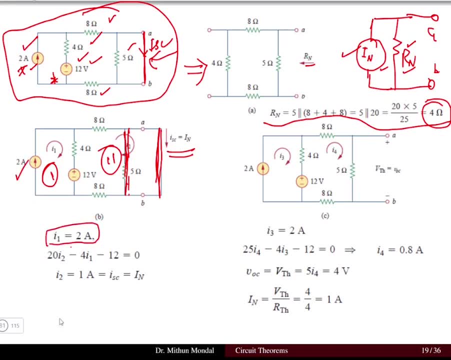 is at the terminal or the boundary is 2 ampere, so that we can get it easily. Now for the second mesh. we can write the equation: 20 I2 minus 4, I1 minus 12 is equal to 0.. Whereas the current I2 which we 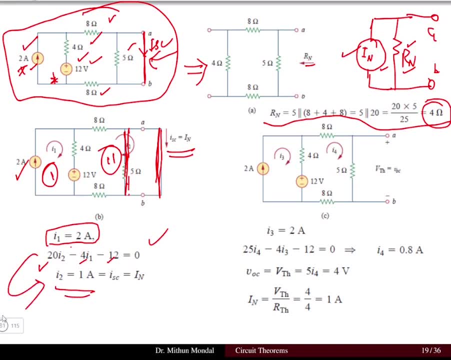 get at 1 ampere from this equation after solving this equation is basically the short circuit current of the norton current. So if we get the short circuit current of the norton current, we have got the norton current. So we have got the value of the norton current as 1 ampere and r. 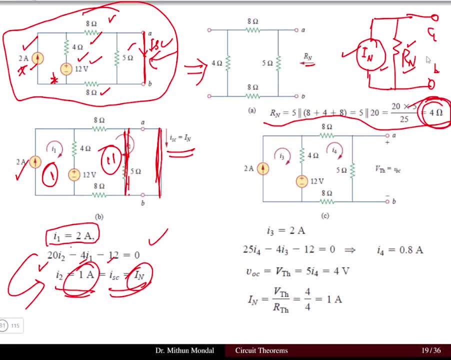 norton is 4 ohms, We can create this circuit and we can obtain anything which is happening at the terminals Now, the same we could have done by some other method. So one alternative method we discuss with the help of Thevenin's voltage. Thevenin's voltage is basically the open circuit voltage at 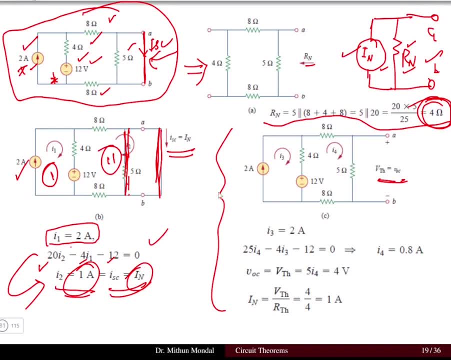 the terminal. So what we do is we take the open circuit voltage at the terminal. So what we do is that instead of sorting the terminal, we keep it open and we solve the mesh services problem again. So here we have the first mesh, and here we have the second mesh. We solve it and determine. 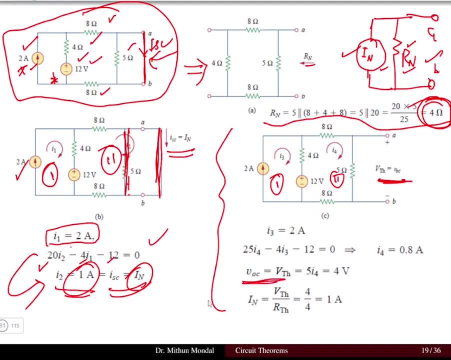 the open circuit voltage, that is the Thevenin's voltage, which we get it to be 4 volt by solving the two meshes. That is the KVL equation of the two meshes. Then, once we have obtained the Thevenin voltage- and r Thevenin and r norton are same- we can obtain the I.